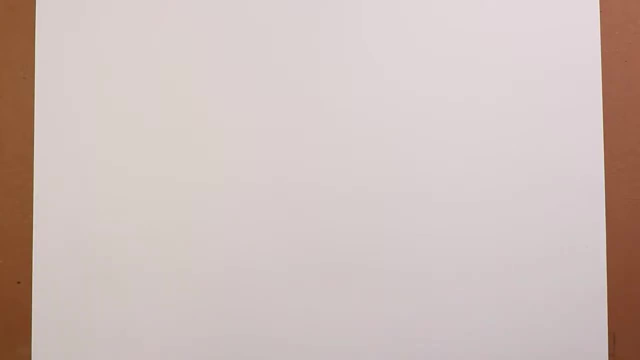 Those are typical sorts of devices, All right. so when we left off, we were talking about a PN junction, like so Our schematic symbol for a diode, because this is basically what a diode is, it's just a PN junction Schematic symbol looks like this and the same orientation. 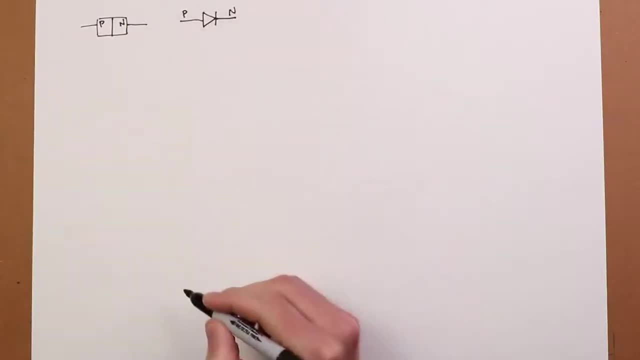 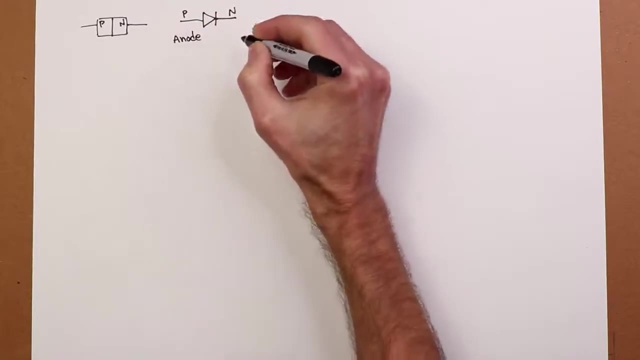 In other words, P material here, N material here. This side is referred to as the anode, This side is referred to as the cap, This side is referred to as the cathode, And it's often abbreviated with a K for a typical barrel style diode. 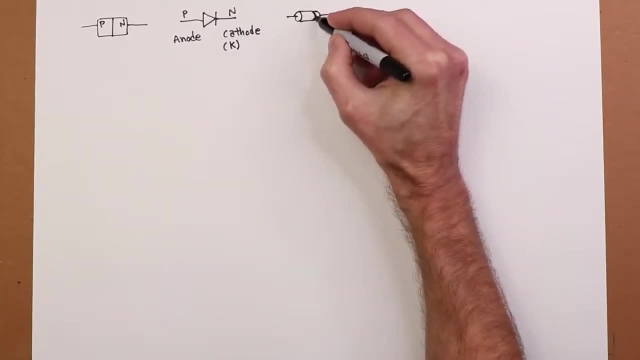 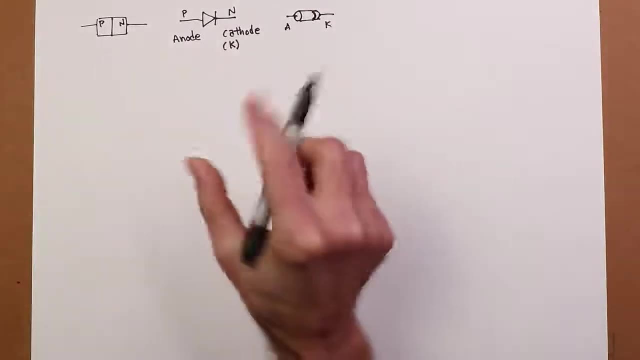 You'll find a band on the cathode. You'll see a little bar out here. All right, so that's the cathode side and that's the anode side. The sizes of these, of course, will vary considerably depending on what the 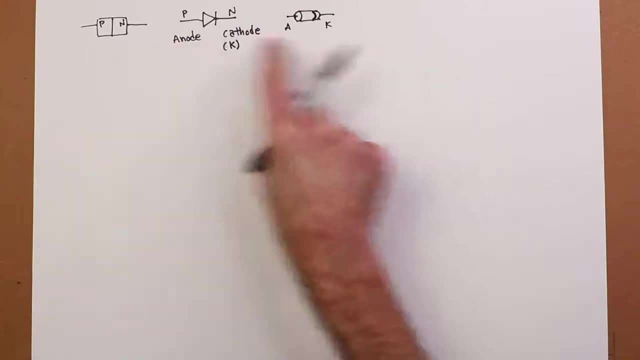 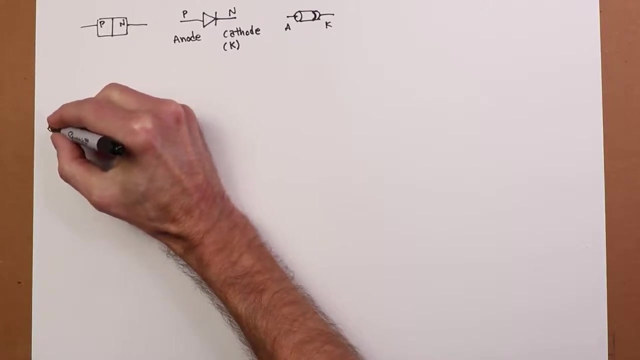 application is. You can generally remember this by saying that the arrow points in the direction of N material or in the direction of easy conventional current flow. All right, So we drew a little diagram, a graph of the operation of our diode PN junction anyway, and it looks something like this. So here's the forward diode voltage, Here's 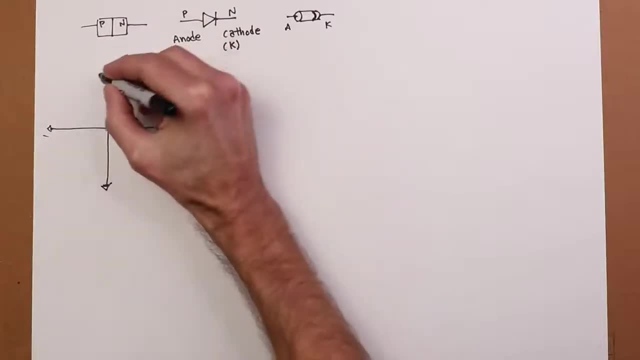 diode voltage And then here's the current. So what we saw is basically no flow until we hit the knee of the curve. Then that thing takes off. That knee for silicon is around 7 tenths of a volt In the other direction, in the reverse bias. 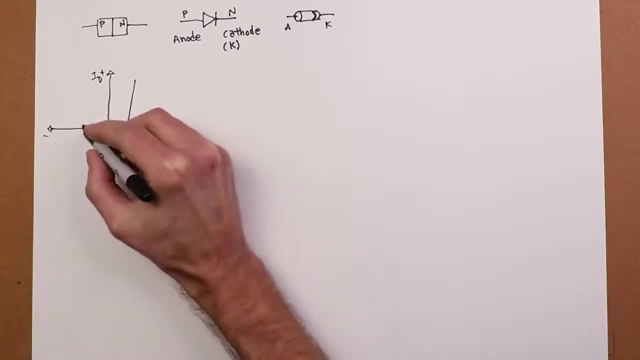 direction. we get no current. If we go far enough- and I'll put a little break here, because this is not to scale- If we go far enough, we will hit breakdown and we'll get a sudden very large increase in current. So this is your breakdown. This is usually 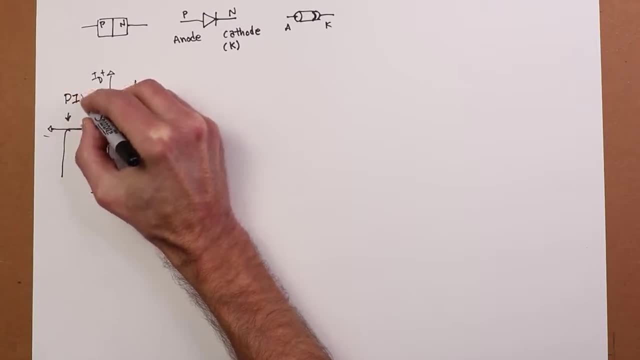 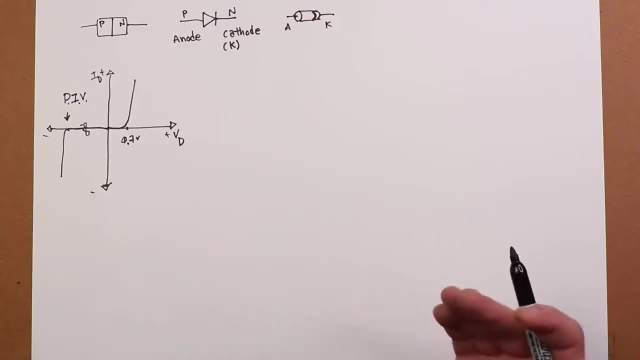 referred to on a data sheet as PIV, peak inverse voltage, And it will depend considerably on the design of the diode. So you know a small signal diode that might be 50 volts, 100 volts. For a large rectifier, you know it might be 400 volts, 600 volts, something like. 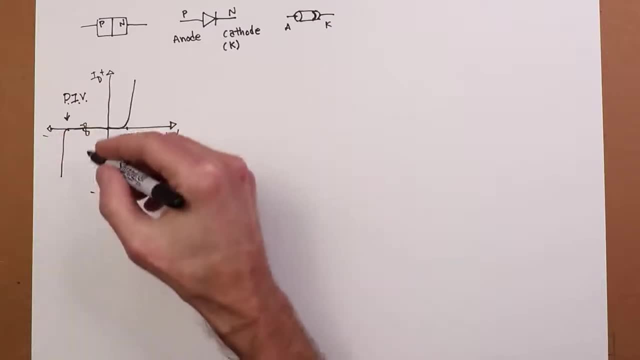 that. So as long as the current is not too high, we'll get a sudden very large increase of potential. The reverse bias potential is less than that. We just treat this as an open. Okay Models, You can think of the diode as simply being a switch. This is your most. 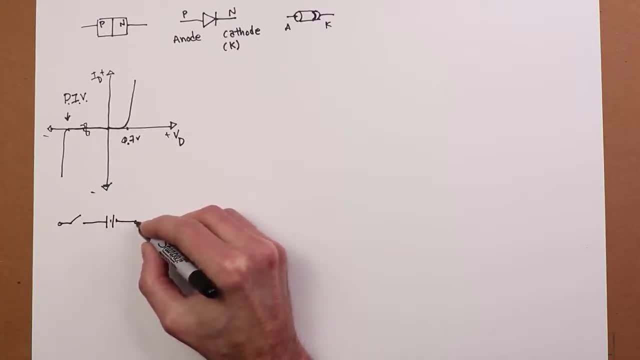 basic model: Simple on-off switch and there's a little voltage. that's the knee voltage. This is your 0.7.. This isn't a real source. Don't think you can hook this up and get current out of it. This is just a little model technique that we might use for a circuit. 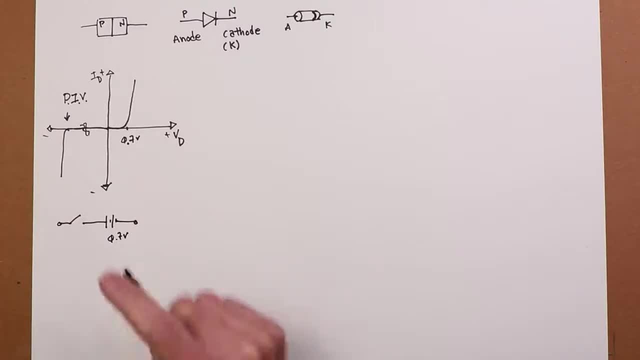 analysis and I'll do a couple of examples of that. All right, So basically, when it's forward biased, switches down and you think, yes, there is a 0.7 volt drop on here, Okay, Because you're going to go this way, This aligns with what I'm drawing up here, A somewhat. 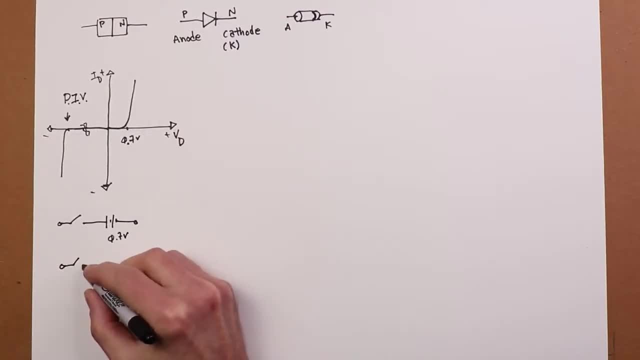 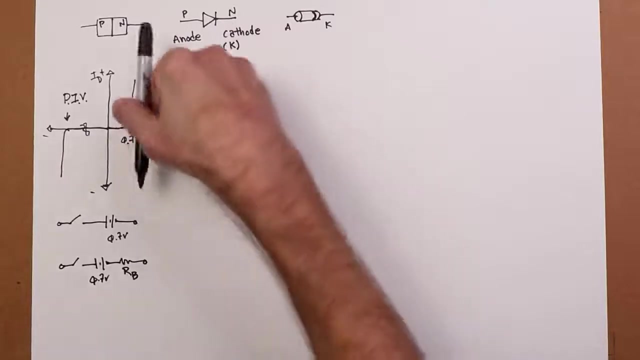 more accurate version of this would include a bulk resistance of the diode, And this is going to give us this little slope that you're seeing here. right, This is not perfectly straight up and down. There is a little bit of a slope to it, So we could model it that. 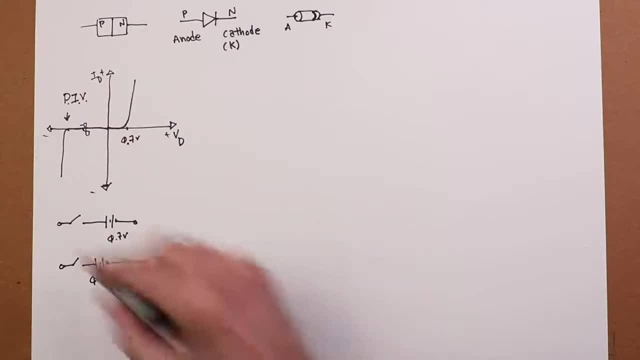 way, All right. Now, given this clearly a non-linear, non-bilateral device, how do we, you know, calculate things like a circuit, current or a voltage, or something like that, Something along that line? So we need to do some examples. Well, the first thing you 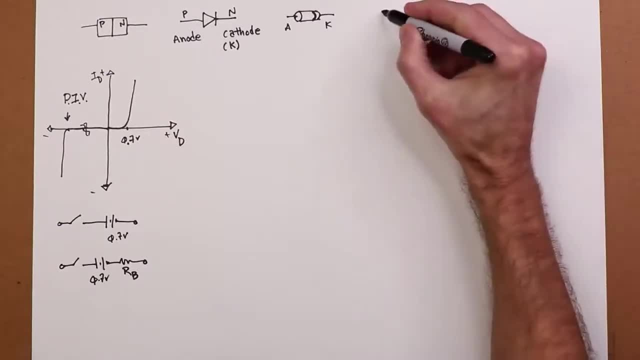 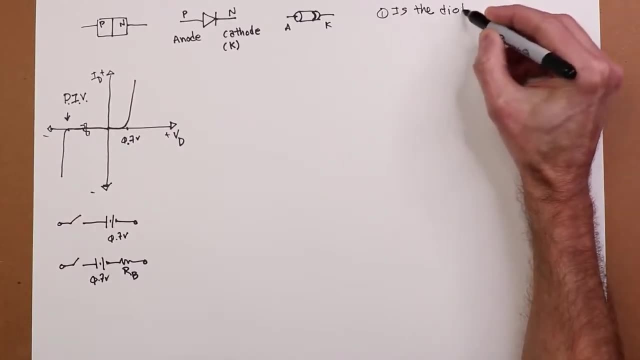 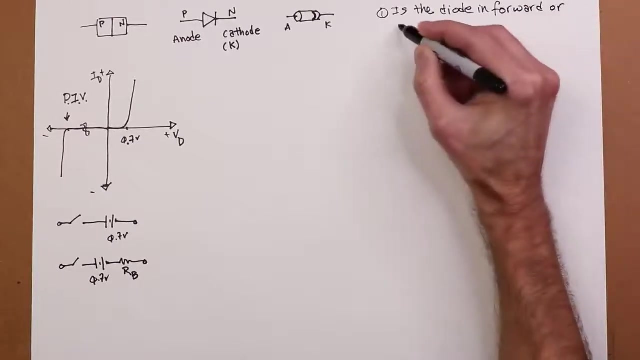 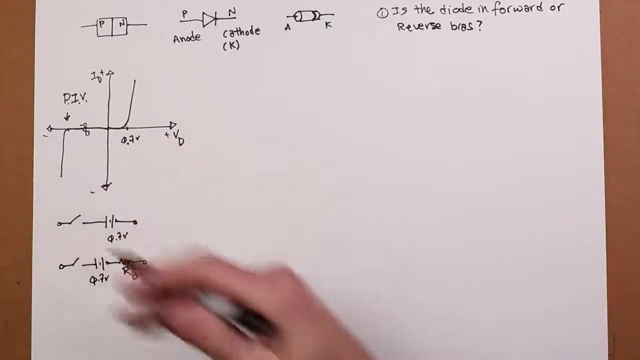 want to do is determine whether or not you have forward or reverse bias. All right, Is the diode forward or reverse bias? Now, once you know the know that, once you can figure that out, then you know whether this switch, so to speak, is opened or closed, And then you can. 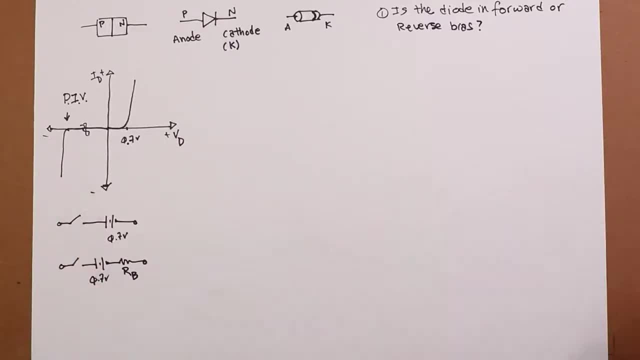 use your approximation here to solve the circuit. Okay, So your second step, in other words, once you know whether it's forward advised, so you insert the model and then simply apply your usual rules, Apply KVL, KCL, Ohm's Law, etc. 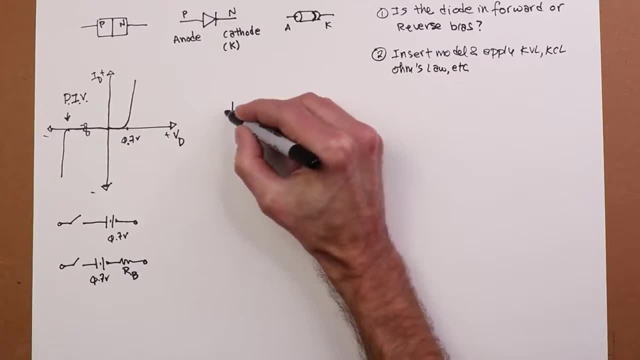 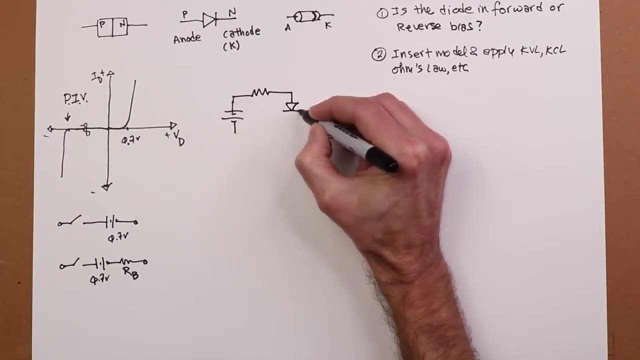 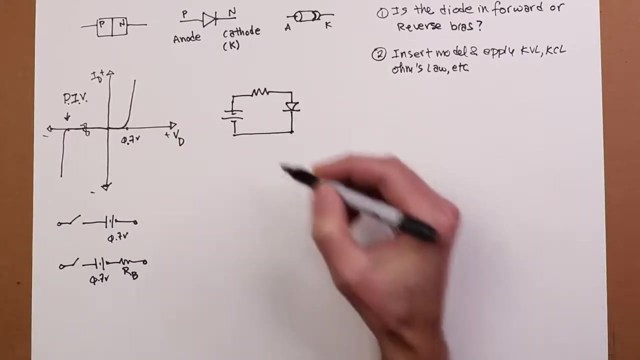 Alright, some quick examples. And I am in all of these examples I'm going to be using a straight silicon circuit Signal diode or rectifying diode, So we can expect the 0.7.. So let's say we have a 10 volt source out here And I'm going to say we have a 1K Ohm resistor. 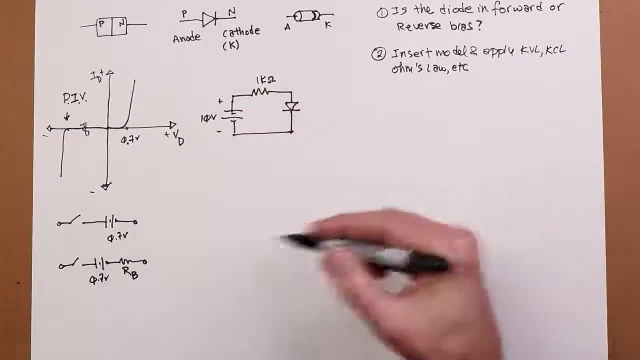 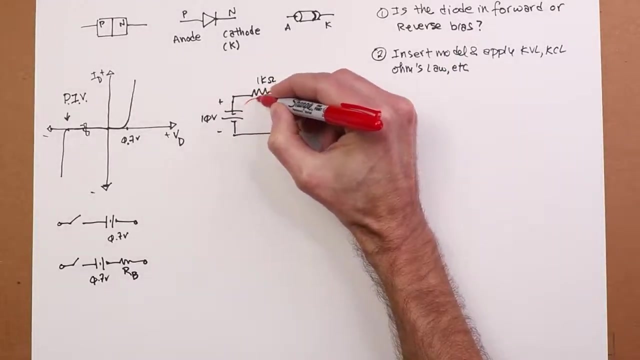 And my question is: what's the circulating current, What's the voltage across the resistor, And so on and so forth. Well, is the diode a forward or reverse bias? Look at this plus and minus on here. I have this single source, So ideally, that wants to create a current like this. 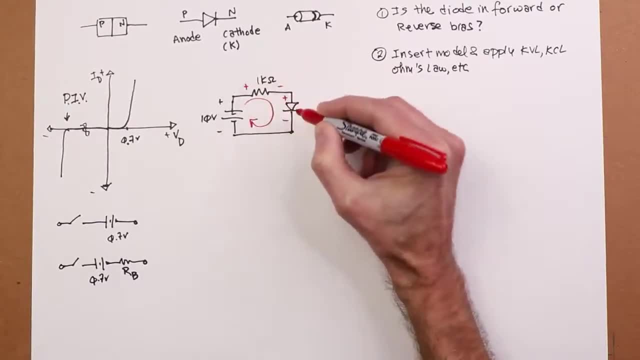 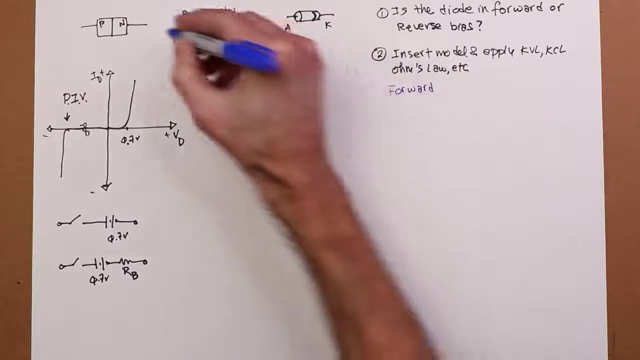 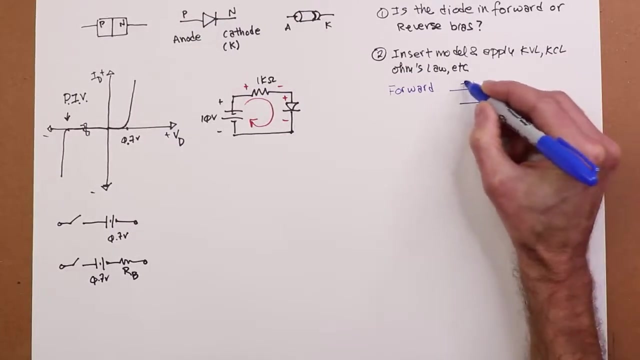 And plus to minus, anode to cathode. that is the very definition of forward bias. Alright, so put a little thing over here. Forward means remember what I said: arrow points in the direction of easy current flow. So your current's going like this. you get a drop like so. 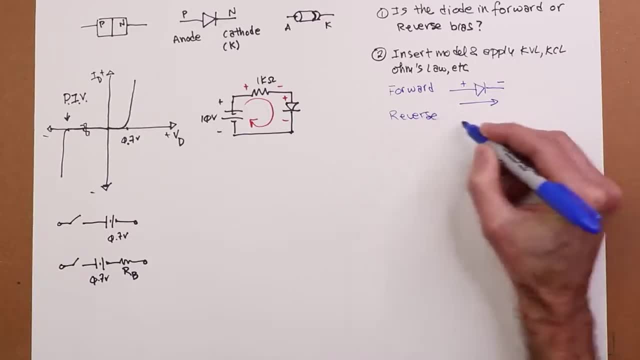 If it's in reverse bias, it's the exact opposite. Alright, so you would have a current trying to go this way, plus to minus that against the flow. In this case, you know this is going to be 7 tenths of a volt. 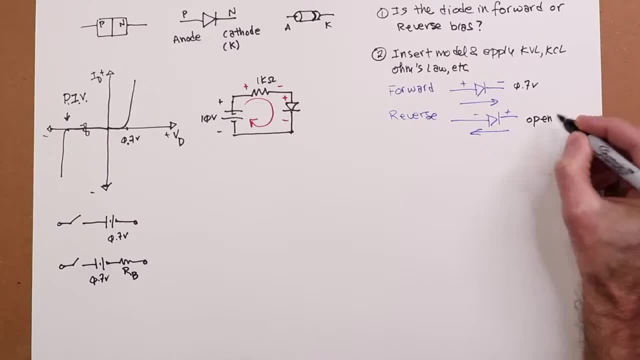 In this case it's an open. So what is the voltage? Well, that's going to depend on, you know, what else is in the circuit, as we'll see. Okay, so in this particular instance, it corresponds to the forward case, right, It corresponds. 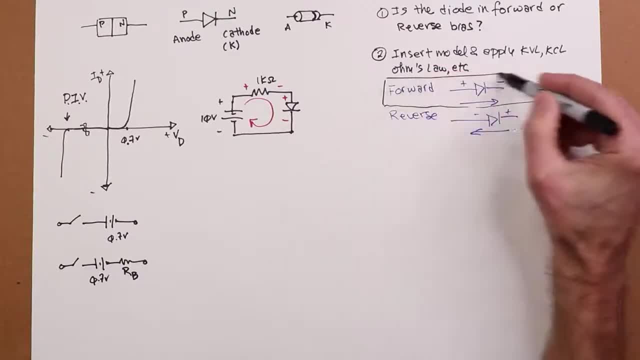 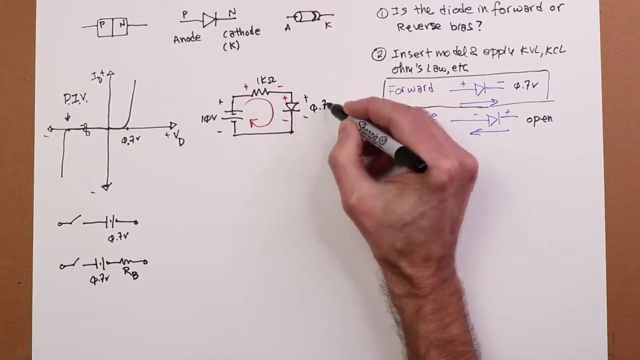 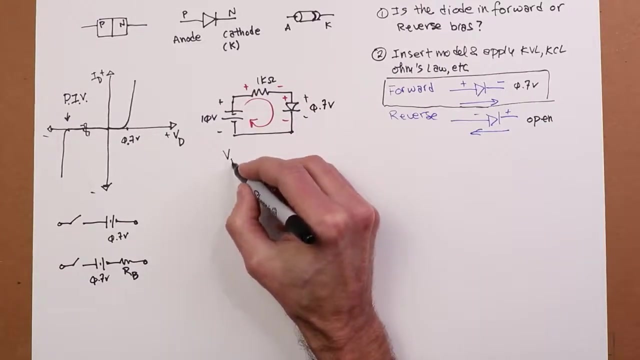 to this guy. So I think of this shut switch 7 tenths of a volt. Now I can apply my rules. If that's 7 tenths, then the drop across the resistor would have to be the source: 10 volts. 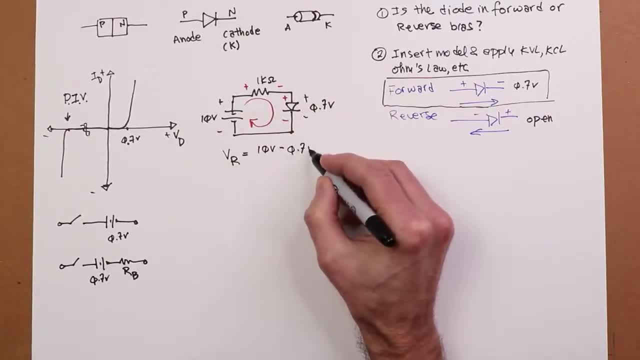 minus the diode. In other words it has to be 9.3 volts And from that we can determine that single current, through Ohm's law, 9.3 volts over k ohm is going to get us 9.3 milliamps. 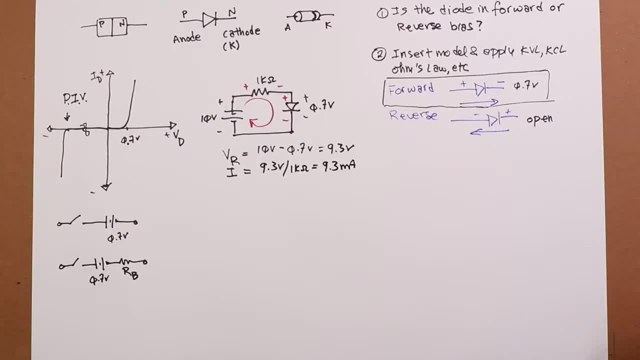 Alright, beautiful. Okay. now what if we flip this? So I'm going to use the same circuit. I'm going to use the same circuit, Okay, And I'm just going to flip the diode around. Keep that 10 volt source. 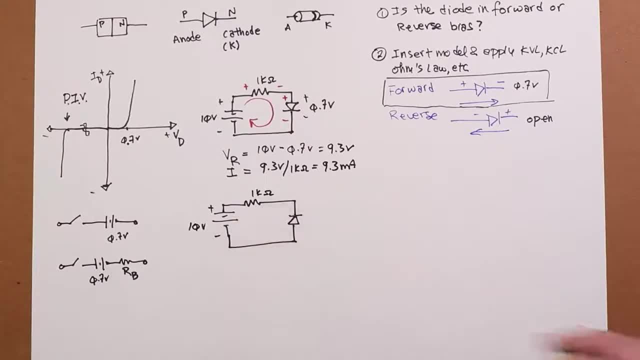 Keep our 1k ohm resistor, Same diode. Now, what do we have? Well, this thing wants to produce a current like this. Okay, What does that give us in terms of, you know, polarities? Okay, 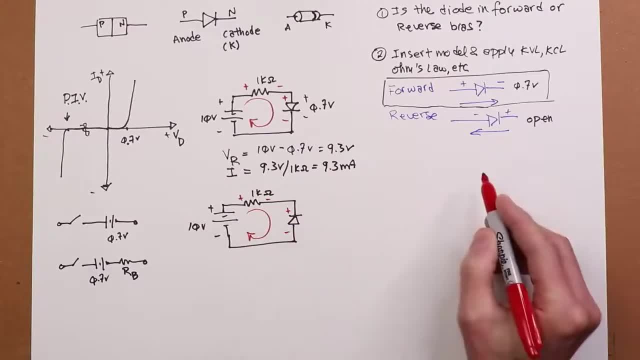 What does that give us? Well, that gives us the diode. Okay, So this is the diode, And I'm going to flip the diode around. That corresponds to the reverse bias case: Right Arrow's going in against what the diode arrow is doing. 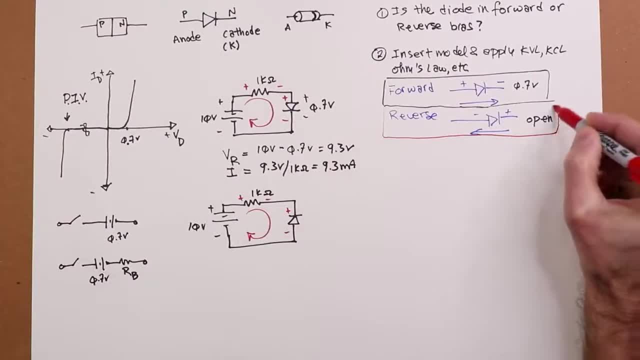 So this is this case. So this is an open. Think of the diode as being an open, Alright, so we've got the switch opened over here, Alright. what do we have? Well, if there's an open, it's just a simple series circuit. 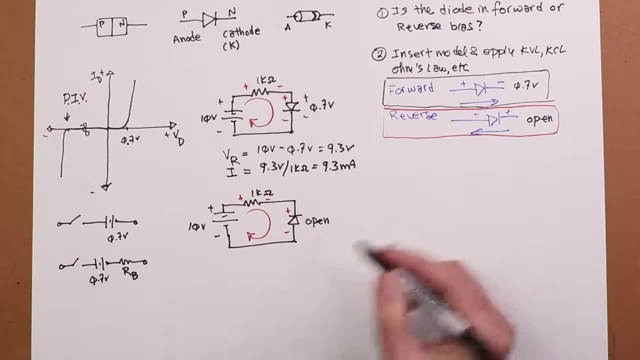 That's it loop right. So if the reverse is open, then obviously the current must be zero. If there is no current, therefore Br is also zero, which means all of the potential from KVL must be sitting across the diode right. Rise has to equal the sum of the drops, So if there 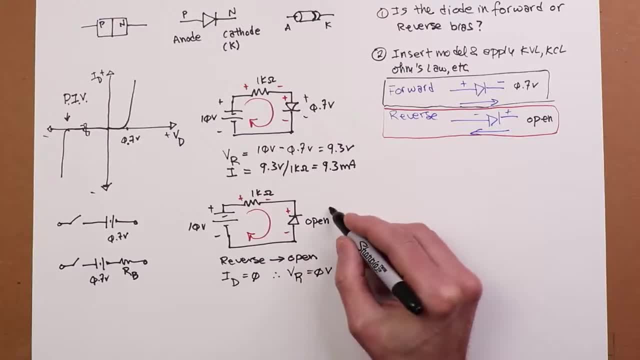 is no drop here, then all of that 10 volts must be sitting across the diode. Now, in reality, there will be a little leakage current. You know this is not zero here. You know there is a real live leakage, but it might be measured in the nanoamps. So you know, with a K-ohm. 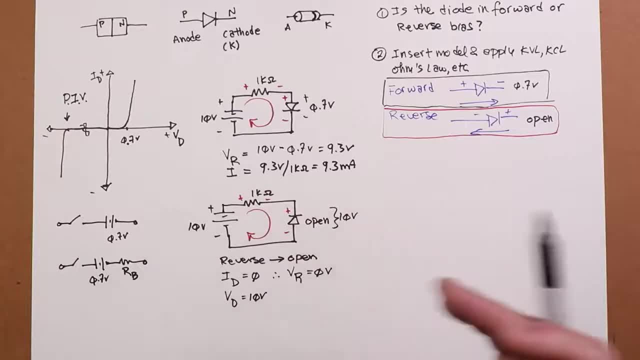 you go in lab with a DMM, you're never going to see it. It's going to work out to this ideal sort of situation that I'm drawing, okay, All right. so forward, reverse, Let's do something a little bit more involved. I'll keep my 10-volt source, but I'm going to put in a couple of 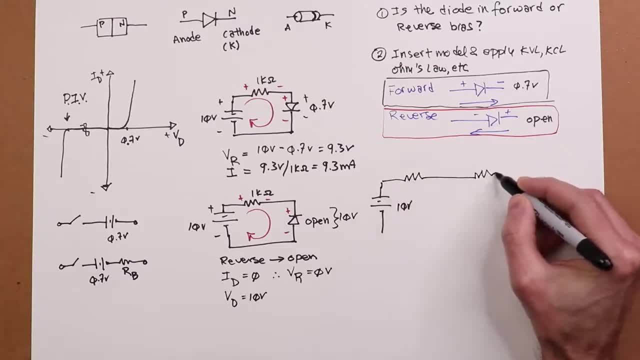 resistors and a couple of diodes, And I'm going to call these, for lack of better names, diode 1, D1, and diode 2, D2.. Now the resistors. I'm just going to make this a 1K and a 2K, So our question would be: you know? 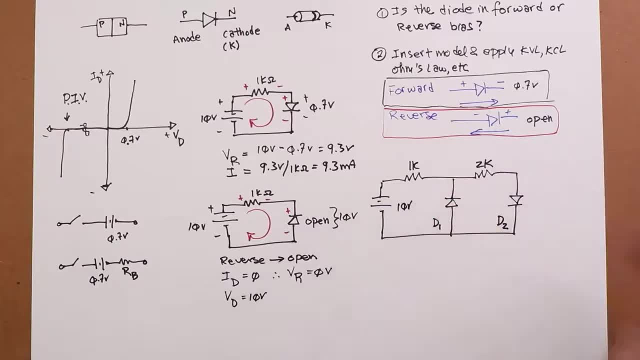 what do I get for? you know, the voltage across the 1K, the 2K, the diodes right, What are the currents that we see? Things like this, Standard kinds of questions. Well, again, ask the question: are these diodes in forward or reverse bias? Well, what would 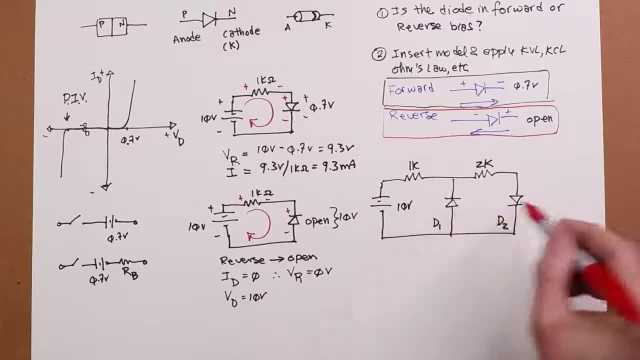 you get from this one source. You know, if you just thought of these for a moment as just being like a resistance, you know some unknown value, where would the currents be flowing? Well, current would go through like this. Then, at this node, it would split right. 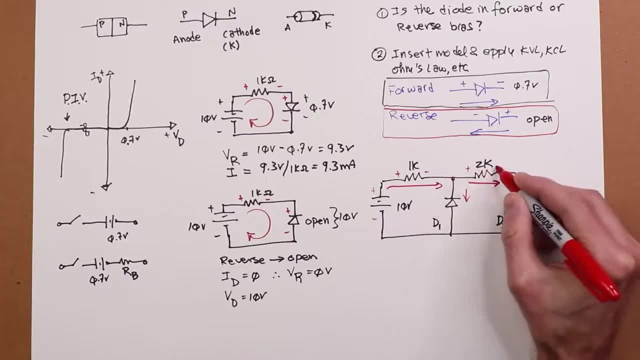 You'd have a current going this way, and you'd have a current going this way. Well, this way, right. that current continues down like this, As does this. So what do we have? Well, D1, plus to minus, which is cathode anode, that's. 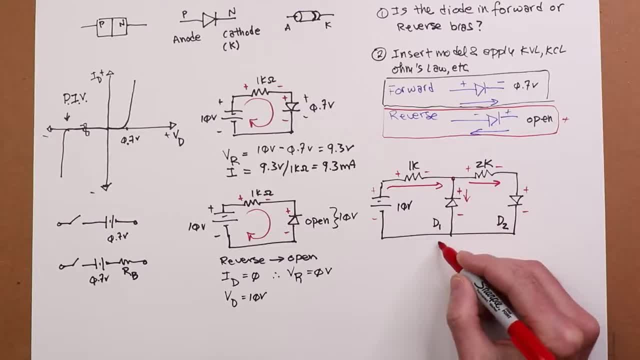 this case right. So this thing is off. This is the reverse case. This one plus to minus, anode to cathode, that's the forward case. This is the on of 0.7.. So we think of this as just being 0.7 volts. Well, if this is, 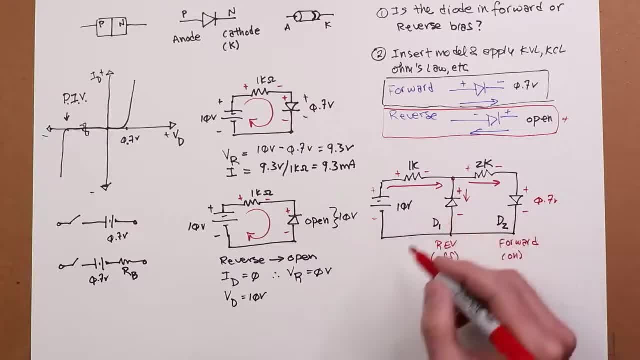 off if this is open. right, you could simply think of this as a source: two resistors and this 0.7 volts, right? Just pretend this isn't even here. So what does KVL give you? right? KVL would say, well, I've got 10 volts. 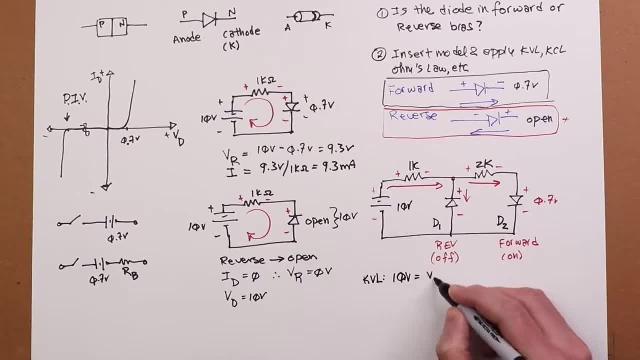 That's got to equal the drop on the 1K plus the drop on the 2K, plus the drop on D2, which we know is 0.7 volts. So 9.3 volts must drop across the 1K and the 2K. Therefore, the current 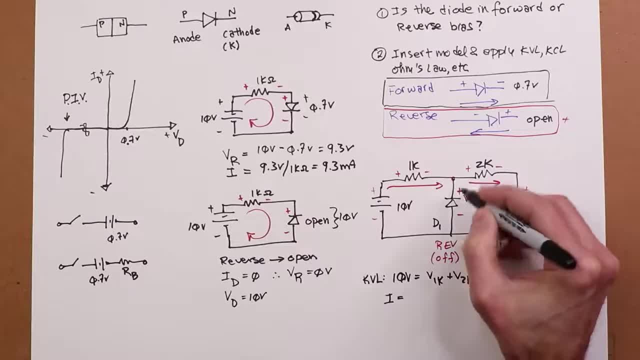 this current, which is going to be the same as this current, because, again, this is an open. we can assume the current through D1 is 0. That's going to be 10 minus the 0.7, 9.3 volts over 1K plus 2K, 3K right. So when you divide that out you're going to get 3.1 mils. 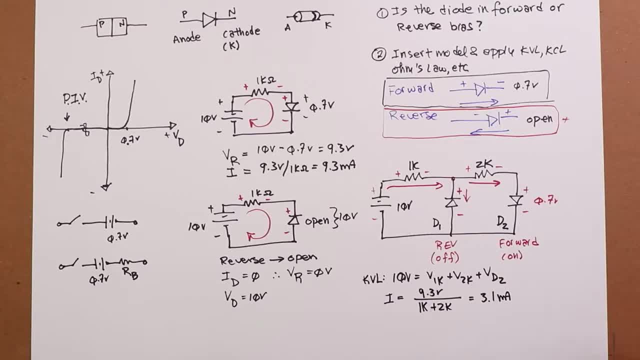 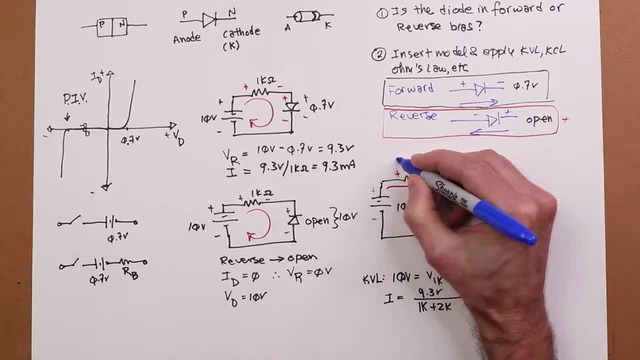 Now you can take that 3.1 mils figure out the drop on the 1K. 1K times 3.1 mils will give us Ks and mils cancel. we're going to get 3.1 volts across this guy. 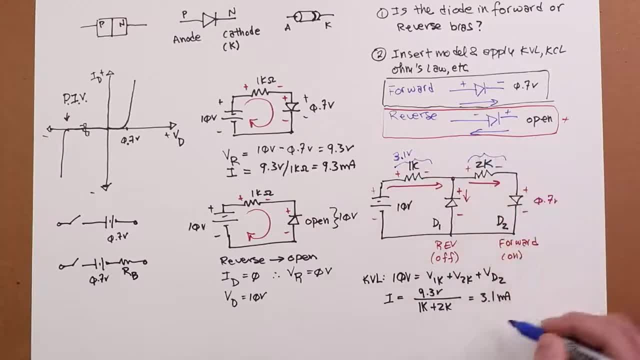 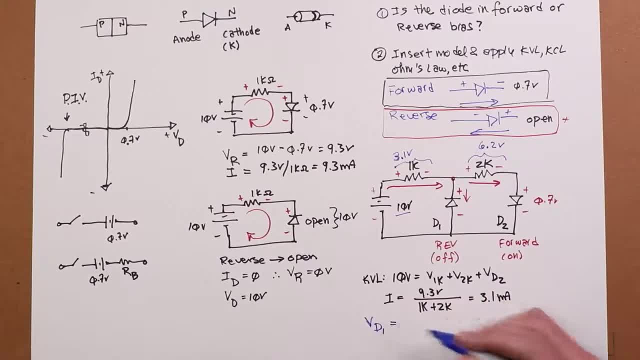 Well, that's from this point to our reference to our ground down here, assuming that's ground. You can find that a couple different ways. you could say: well, we start with 10, we drop 3.1, that's what's left- 6.9. or you could say: this is: 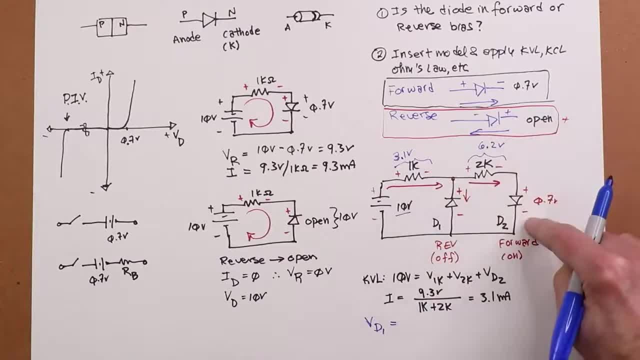 equal to the parallel combo over here, which is 6.2 plus the 0.7, either way, 6.9 volts. okey, doke, beautiful, all right. last question: what do you get if you swap orientation of these two diodes? in other words, what would you get if you put d1 in this way?